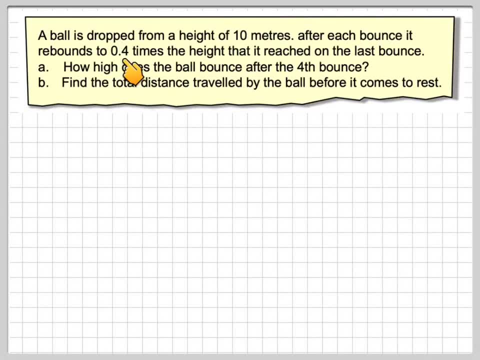 A ball is dropped from a height of 10 meters. after each bounce It rebounds to 0.4 times the height that it reached on the last bounce. How high does the ball bounce after the fourth bounce? And then find the total distance traveled by the ball before it comes to rest? 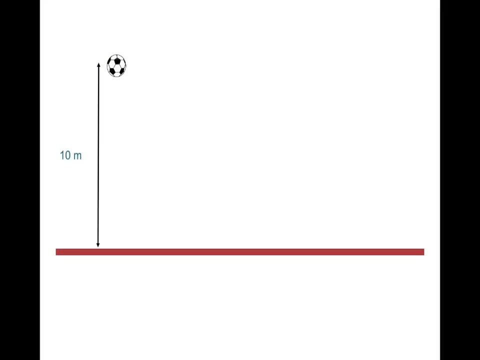 Okay, so just before we do it, let's have a quick look at this animation. So basically, we've got a ball and what it does is we drop it and of course, it's going to bounce, bounce, bounce, bounce, bounce. So the path will look roughly like this: It will start here at 10 and go down, come up 0.4 times of. 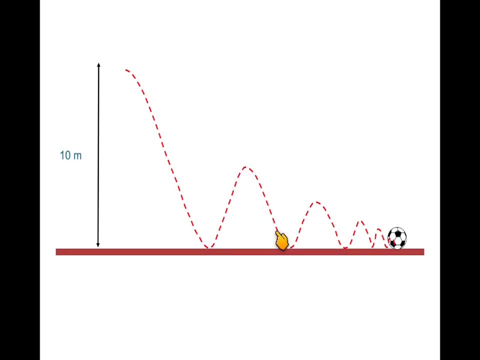 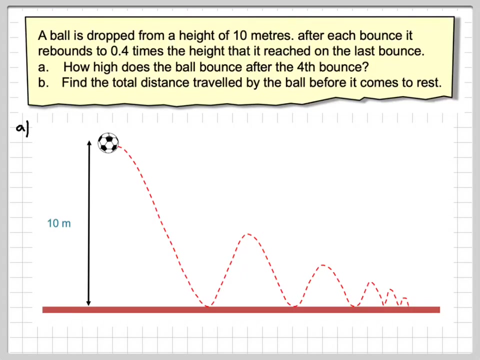 10.. So this one will be 4, and then 0.4 times of 4, and then again like this: So this height here, this height here and this height here and this height here, and then so on, will form a geometric sequence. So let's have a look at this diagram here. So here we have the diagram. So this, the 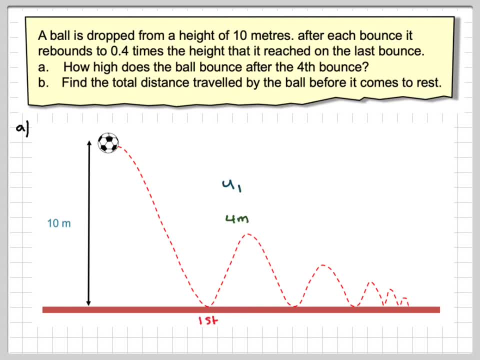 first bounce is here. Okay, so the first term of this geometric sequence will be 4 meters, which is point four of ten. The next one will be four times zero point four. So this will be be 1.6 meters, this height here, and then the next one will be 4 times 0.4 squared. 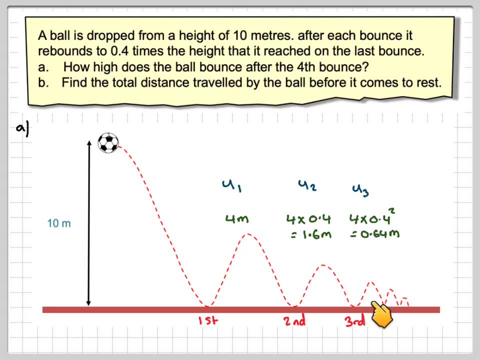 which is 0.64. so this one will be 0.64. and then this is the fourth bounce, and we have to find this height here, but the sort of general term of this geometric sequence, un is going to be the first term, which is 4 times 0.4 to the n minus 1.. notice that the first term is not 10. 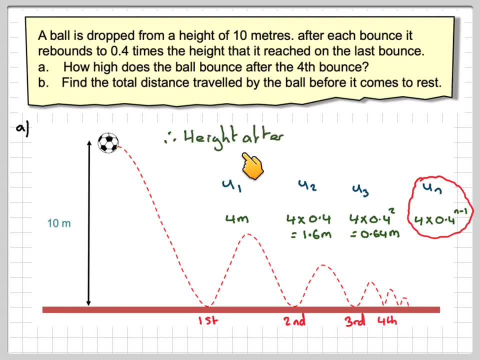 we'll look at that in a minute. so the height after the fourth bounce will be equal to 4 times 0.4 of 4 minus 1, which is 3, so 0.4 cubed, which is 0.256 meters. right now we need.